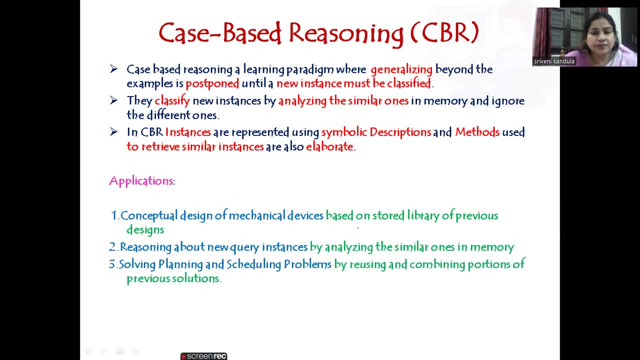 on that the reasoning for the new instance can be given. The third application is solving planning and scheduling problems. So for this we can reuse And combine portions of the previous solutions. Suppose, if the entire solution is not matching, if some part is matching also, so from one. 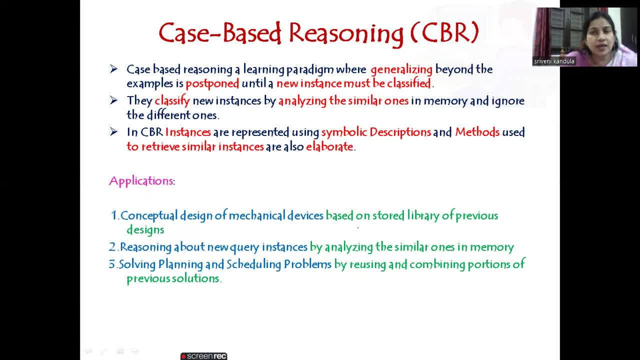 solution, we can take one part and from the other solution we can take other part and finally we can combine all those. So these are the applications. So let us discuss one example, that is, the CADET system, which is a prototypical example. 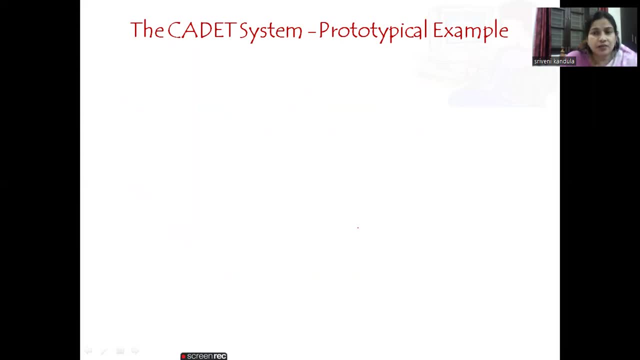 Okay, This is just a prototype. It's not an application, It's a final design. It is just a prototype. Okay, So here the CADET system employs CBR, case-based reasoning to assist in the conceptual design of mechanical devices. 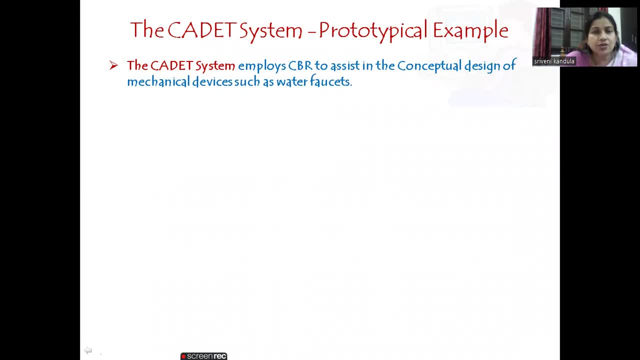 So this is the first application we are talking about. So here, what is the application we are talking about is the design of water facets. Here you can see the example. So here we already have a stored case which is a T-junction pipe. So you can see the structure of it and the function to describe. 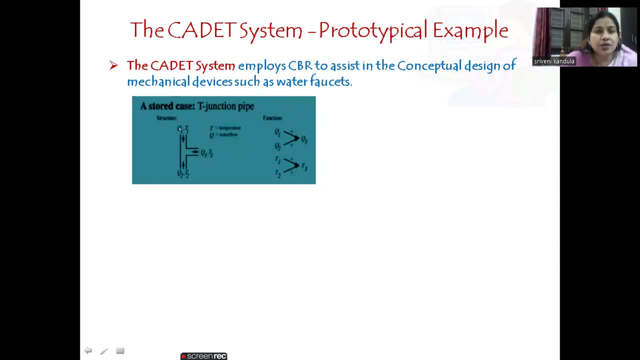 this structure. So this is the structure. So here you can see: Q1 is the water flow, T1 is the temperature. So Q1, T1, Q2, T2 are given as inputs and, based on that, an output- Q3, T3- is. 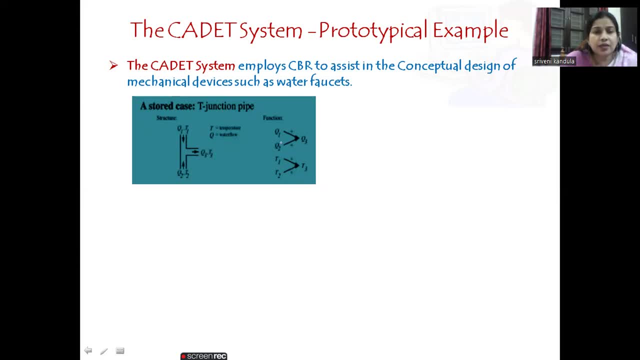 provided. So here you can see the description of it: Q1 and Q2.. So these are the water flows. Okay, so whenever you can see the plus symbol on the arrows, okay, that indicates whenever the water level- Q1, Q2- is increasing, Q3 will also increase, Similarly T1 and T2.. So here you can. 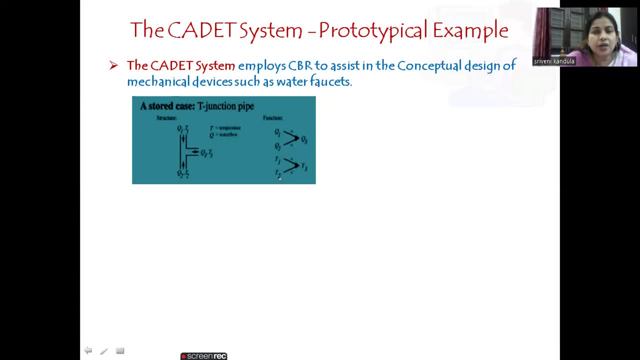 observe a plus sign which indicates whenever T1 and T2 are increasing, T3 will also increase. Suppose, if you have a minus sign on this, okay, so the corresponding output also will be reduced. Okay so whenever you see a plus, that means Q3 will increase with the increase in Q1.. 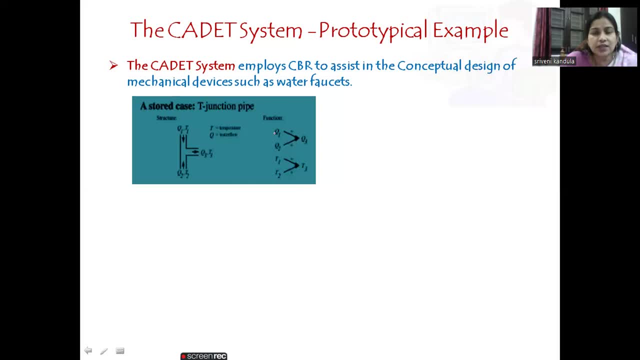 If you see a minus, Q3 will decrease with a decrease in Q1.. Okay, so this is one stored example. So now let us see how to apply this for a new situation whenever it is asked. So here you can see. the function is represented in terms of qualitative relationship among the. 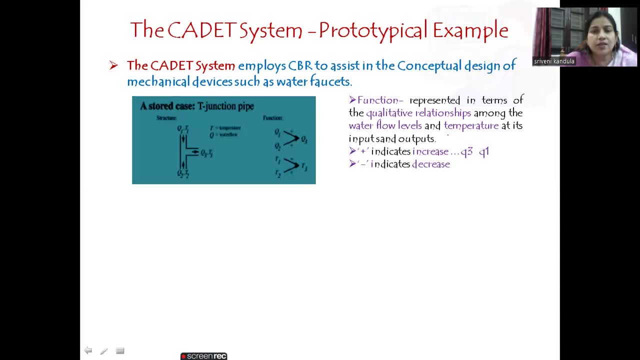 water flow and the temperature. So these are given as inputs and outputs. Okay, plus is indicating the increase and minus decrease, as we discussed. So now this CADDED system. it contains a library which has 75 previous designs, And here each instance stored in memory is represented by describing both its structure and its 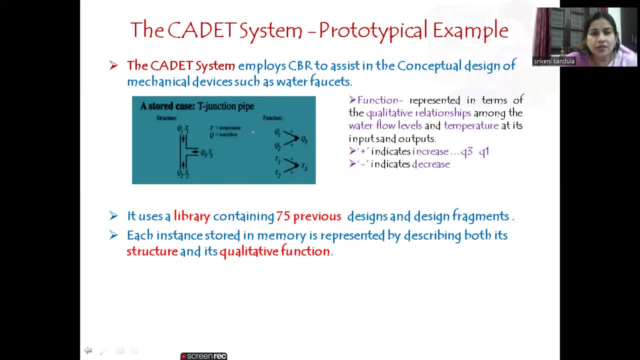 qualitative function. For all these 75, here we are. we are seeing only one example Like this. totally 75 examples are already stored, 75 designs are stored. For each one we have a structure as well as the associated function. So now, whenever some new design problem is, 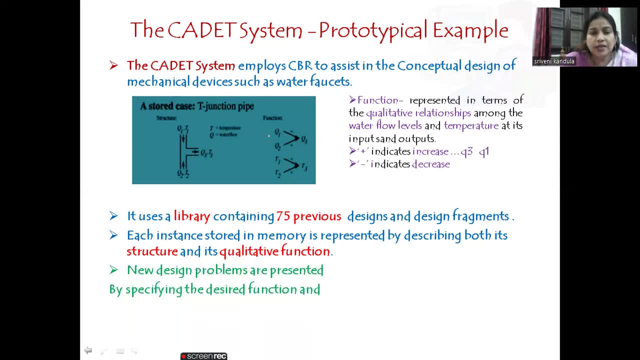 presented. So then, how to solve this? So, that is by specifying how they represent this new design. problem is by specifying the desired function. Okay, So they know what should be done for every design. Whenever some requirement has come, we definitely know what has to be done, what should. 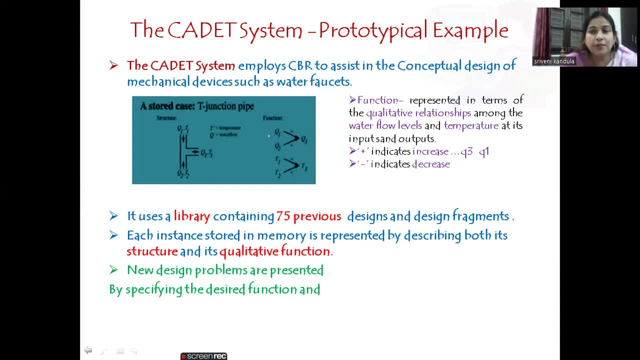 be the outcome, but we do not know how to obtain that. what should be the structure, or what should be the design, or what should be the prototype for that? Okay, So now from the problem. So this is a backward propagation. we are doing So here. we know the solution means we know the. 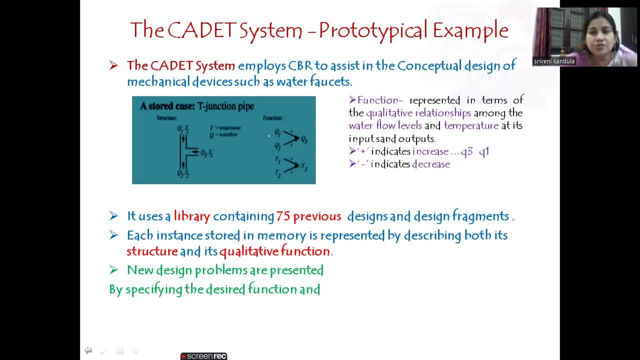 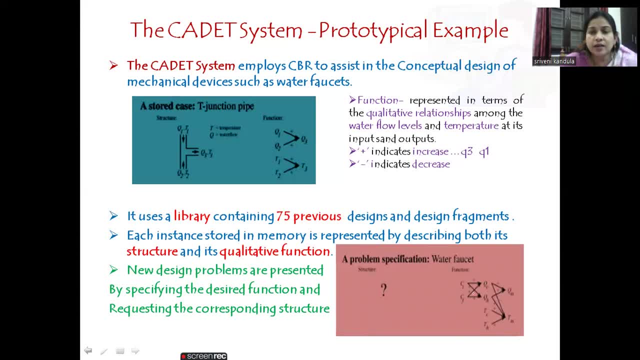 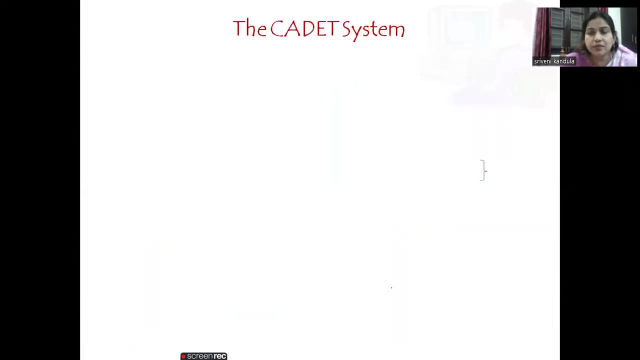 given. So here the function is given. So for this function, what should be the structure? Okay, So this sort of new problems will be given. So now, from the CADDED system, a solution should be provided for this. So now here, if you observe this water faucet problem, 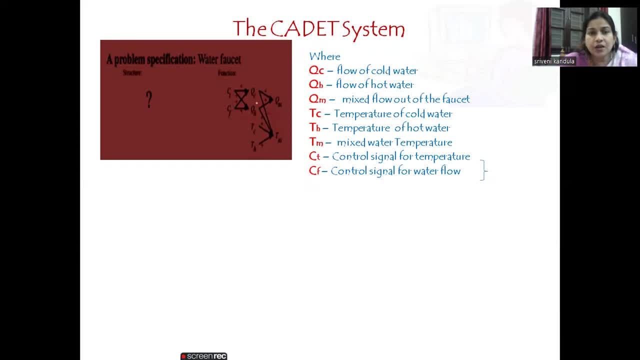 here we have Qc and Qh, which are flow of water and hot water: c for cold water and h for hot water. similarly, tc is the temperature of cold water, th is the temperature of hot water, qm is the mixed flow, mixed flow of this cold plus hot water. 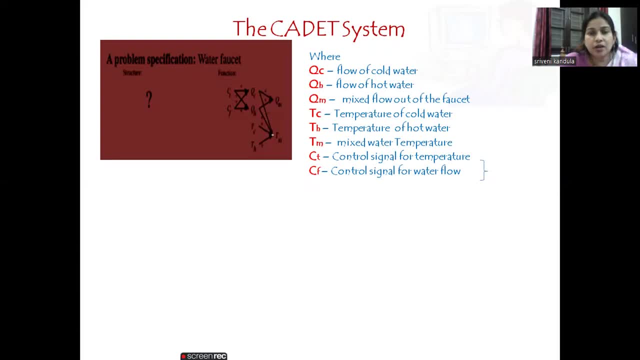 whereas tm is also the mixed water temperature. so okay, here it is taking cold water temperature as well as hot water temperature and flow of the cold water and flow of the hot water. all the four parameters it is taking into consideration, and mixed water temperature is given and we have two control signals also: ct and cf. ct is the control signal for temperature. 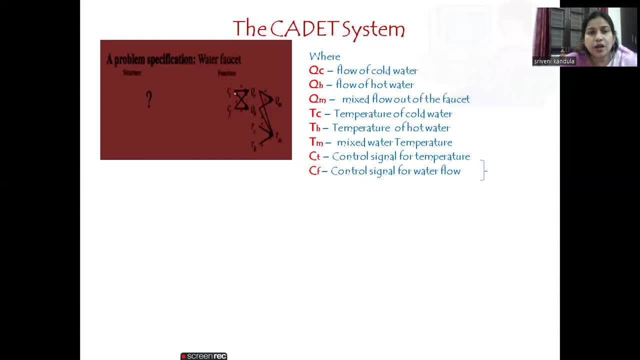 and cf is the control signal for water flow. so these two are controlling qc and qh. indirectly they are affecting qm and tm. so for this the structure has to be provided. so now, if you observe how to solve this, so that can be done in four phases. the first phase is retrieve and reuse, so from the cadet system, from all the 75. 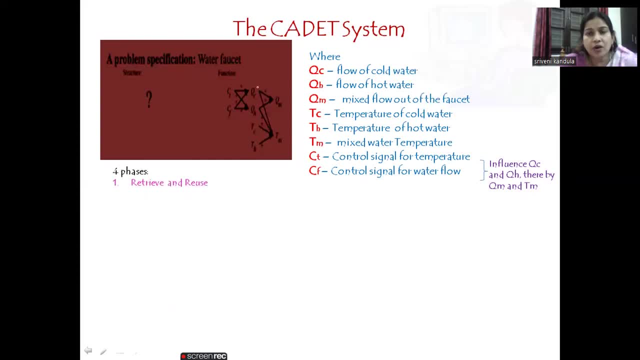 okay. so first of all, we have to retrieve: is there any model which is matching with this and use. use that. okay, already some stored model is there so that we are, we can reuse so in this process, the cadet system it searches for, such as the library for the stored cases. so then, 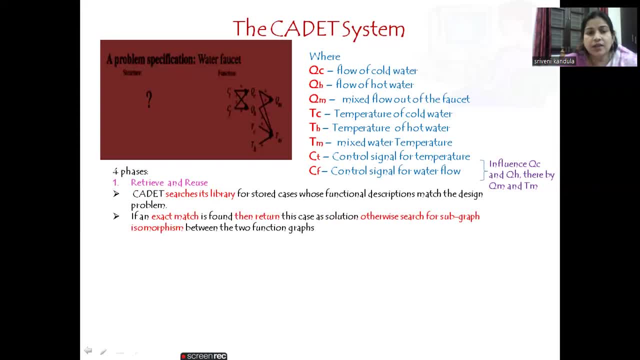 if an exact match is found, then return that case as a solution. otherwise, search for a subgraph. isomorphism: okay, so is there any particular part matching with this particular one? so, for example, if you observe only this particular part, okay, ct2 qc and cf2 qc: okay, so this we can compare with. 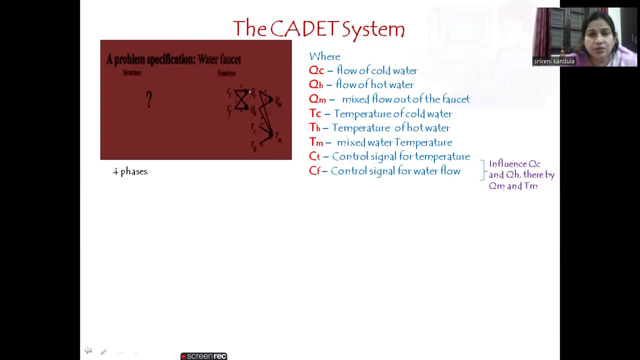 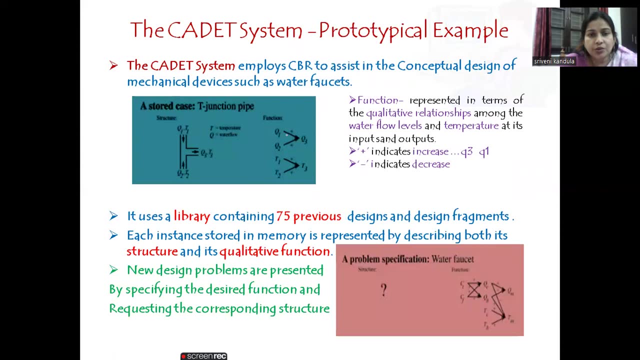 the previous functional description one second. i'll just show the previous slide. okay, so q1 and q2- both are resulting in q3. similarly, t1 and t2 are resulting in t3. so if you compare this with this particular description, okay, so they are matching here. 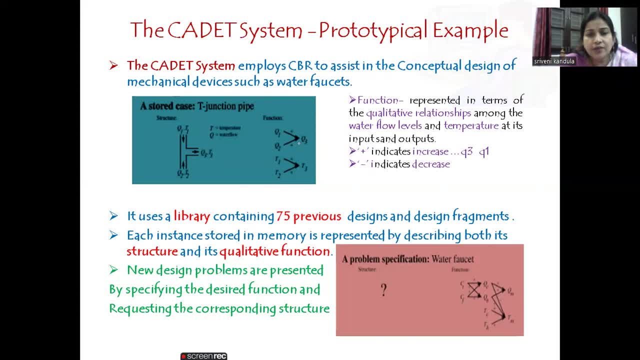 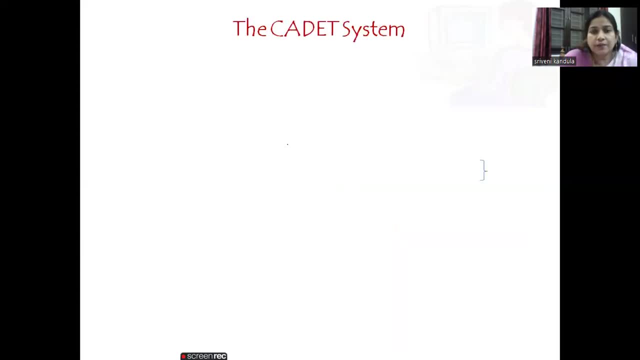 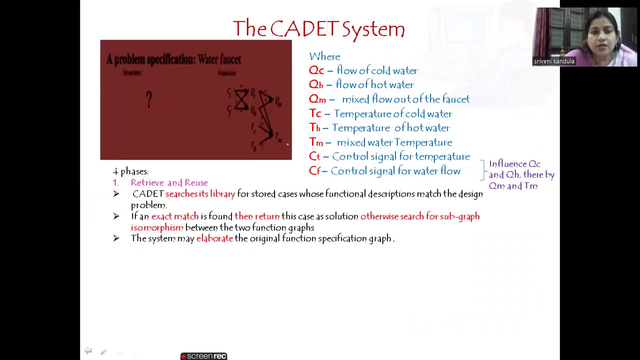 okay, a particular part. so like this it will be checked for sub graph isomorphism or any part of the graph. is it matching with qt, the existing prototype? So in this particular process the system might elaborate also. in some cases the original function specification can might be elaborated also, For example: 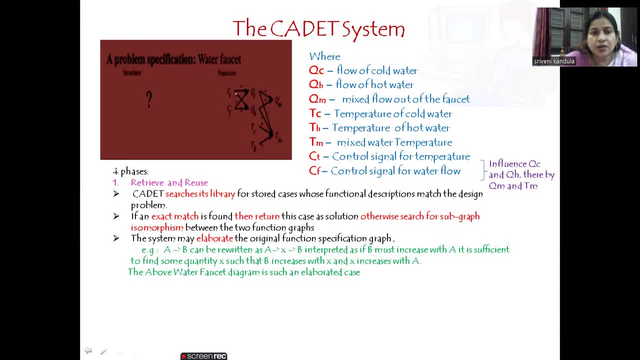 if there is a relation, A tends to B. So here you can see CT is indirectly affecting QM, right? So in between what we have, we have QC which is operating this or indirectly affecting QM. So this can be written as: A tends to X, X tends to B. So this is read as: B must increase. 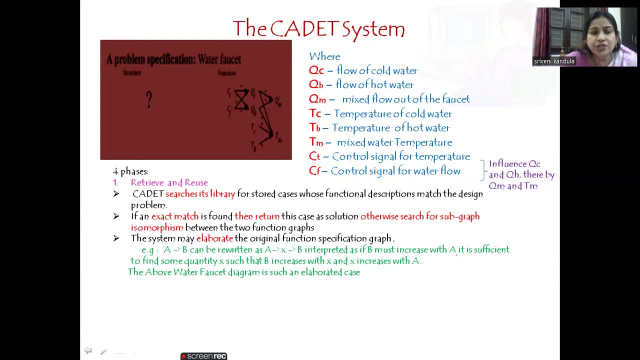 with A. in order to increase like that, it is sufficient to find some quantity X, such that B increases with X and X is increasing with A. So that means here, if we elaborate Ct implies to QM, Let us take the relation as CT implies to QM. 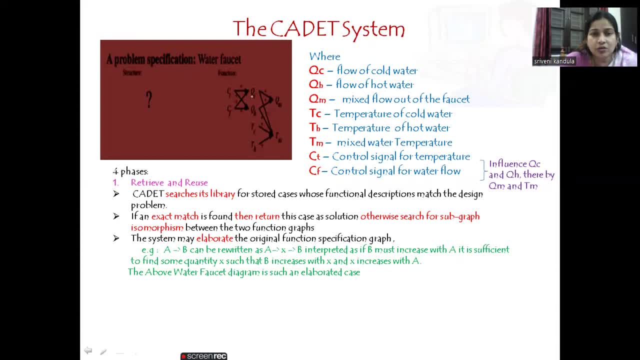 So then, what should be done? QM is dependent on QC. Again, QC is dependent on CT. So that means, in order to increase QM, QC has to be increased, and this QC will increase based on Ct. The next one is merging, So now only. 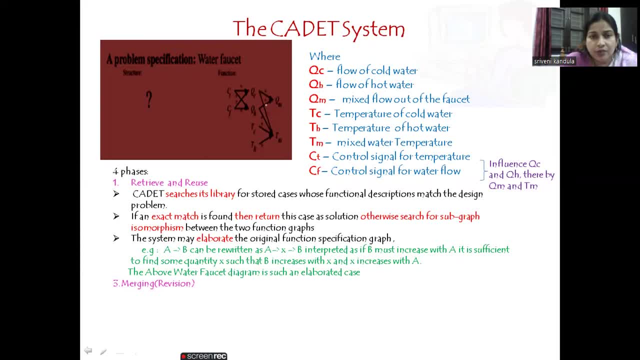 one particular part i have found. so the second case, if you observe here, tm is dependent on qc, which is a negative value. it is also dependent on qh, which is positive, tc and th, so now i have four inputs. okay, so the previous tk or t junction case: it is having only two inputs, so now i have altogether. 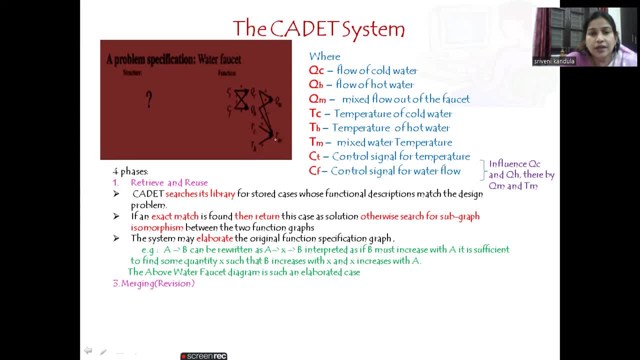 four inputs which are affecting this tm and, in turn, this qc is dependent on ct and cf qh is dependent on cf. so for this, another model should be searched where, if there is already an existing model which will be mapped, which will be matching with this particular case, that means the subgraph. 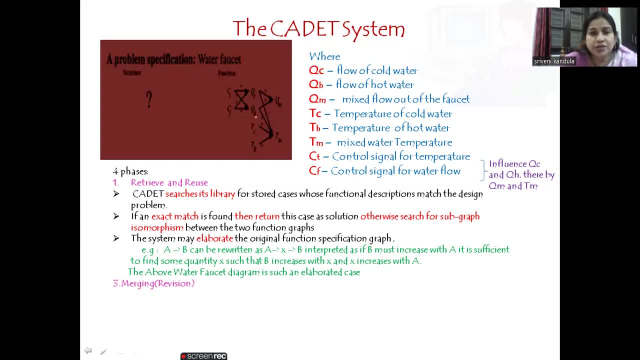 isomorphism. if it is matching, so then that should be retrieved and then these two inputs, which are affecting this tm, which are affecting this tm, which are affecting this, should be combined. so that is what meant by merging or performing a revision. so while merging like this, sometimes design from the first principles must be done, sometimes there. 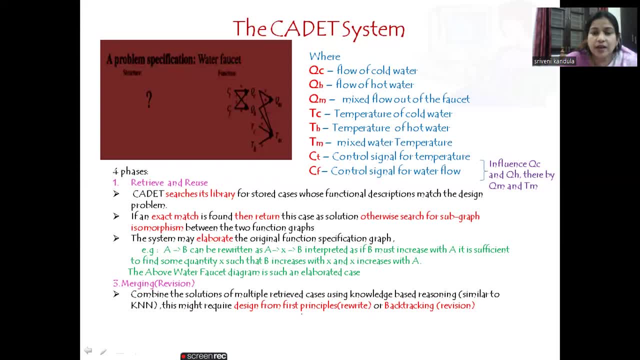 is no matching case. in that case, what should be done? again? it has to be done from the first principles. that means you are newly rewriting everything, or sometimes you might find a some parts as matching. okay, so here in this case, if i see this tc and th, these are matching with. 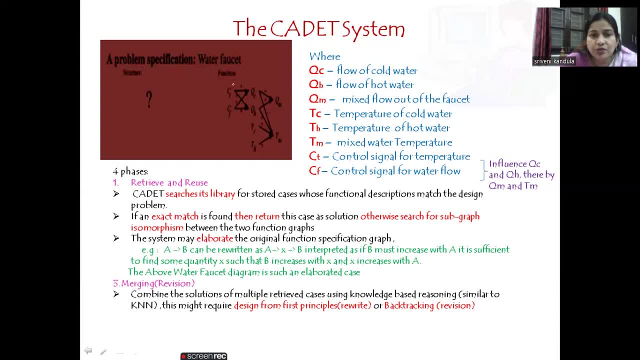 the first case. but when i found this- qc and qh, which are dependent on ct and cf, it is not matching. so what i have to do, i have to back propagate. so for whatever structure i have designed, so that again i have to back propagate and do it again, okay, so this is done using knowledge based reasoning. 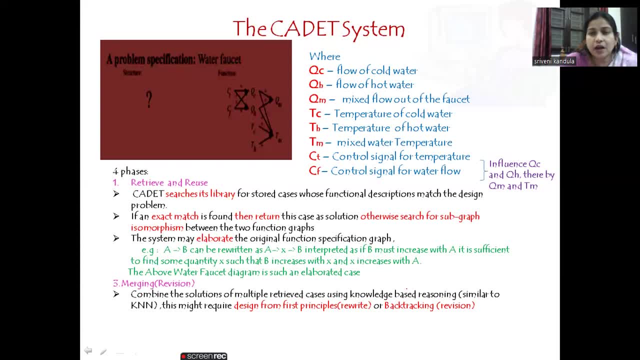 in knn, how we have. we are taking the nearest neighbors k nearest neighbors, how we are taking in the same way. so here we will be using a knowledge based reasoning. okay, from two, three models, we will be obtaining those knowledge and based on that we will be combining the solutions.